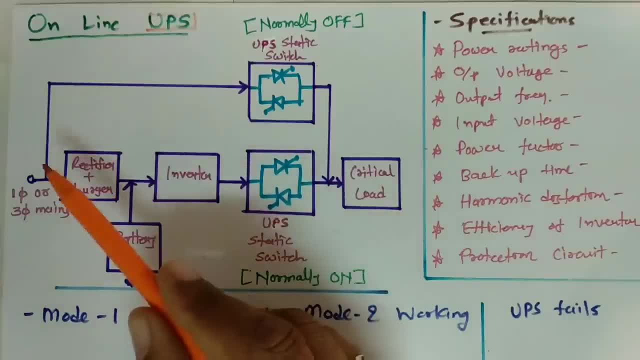 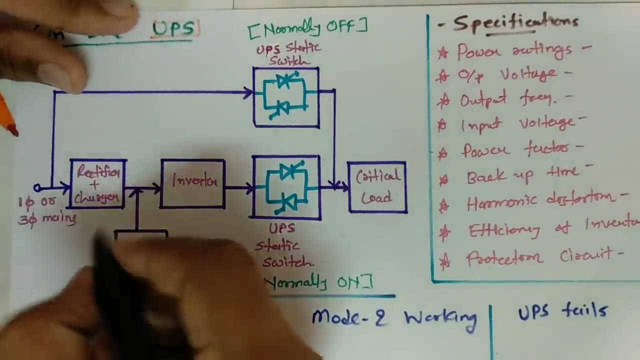 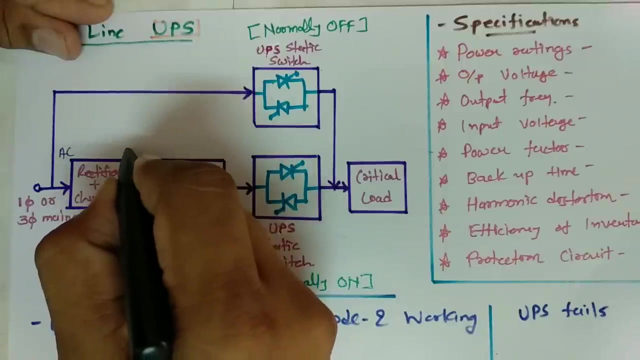 offline UPS, where here we have one phase or three phase power supply that is being given to rectifier circuit and that rectifier circuit is giving DC output. So ultimately, here, at input of rectifier, AC input is there and output of rectifier that is DC. 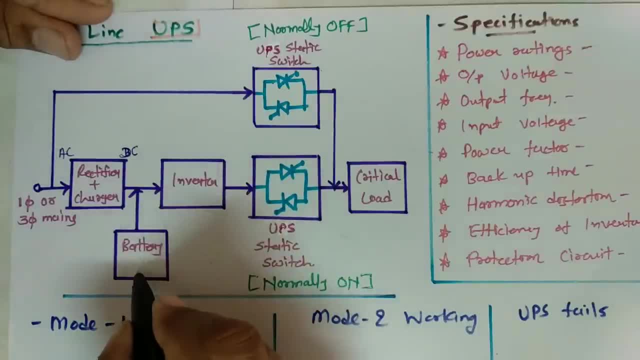 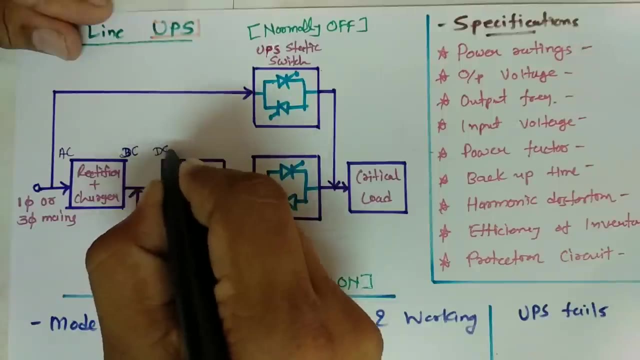 Now this DC signal that is being utilized to charge the battery. So here DC signal of output at rectifier will be utilized to charge the battery as well. as that could be given to inverter. So input of inverter is dc and inverter converts dc into ac. so output of inverter is ac, then after: 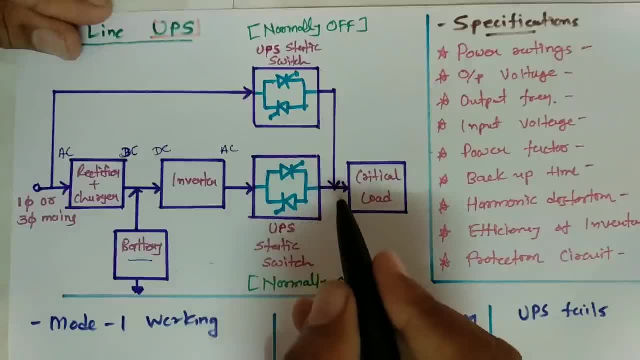 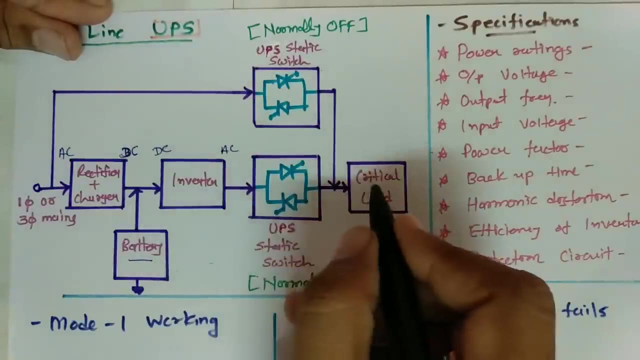 there is ac static switch. so this is what ac static switch that is thereafter inverter and that is what connected to critical load, and one ac static switch that is connected from three phase mains. so, ultimately, ac signal that has been given to critical load. but when we talk about online ups, the basic condition of online ups is this: static. 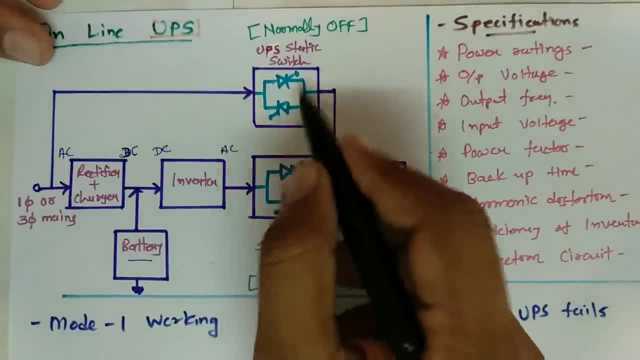 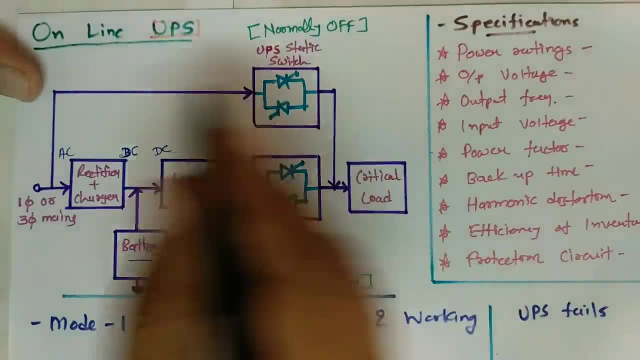 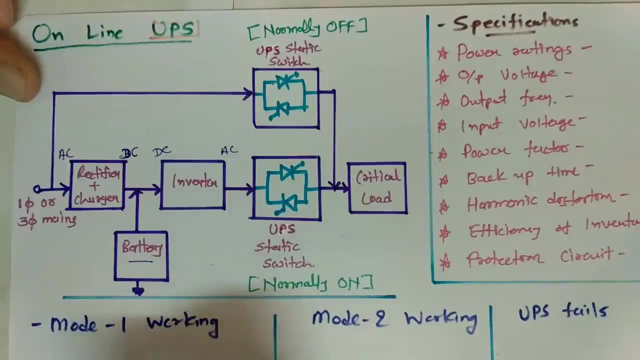 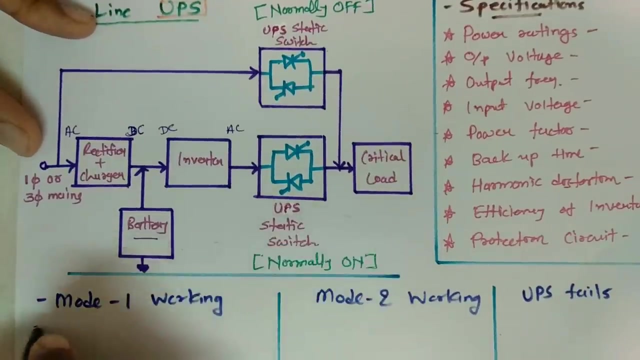 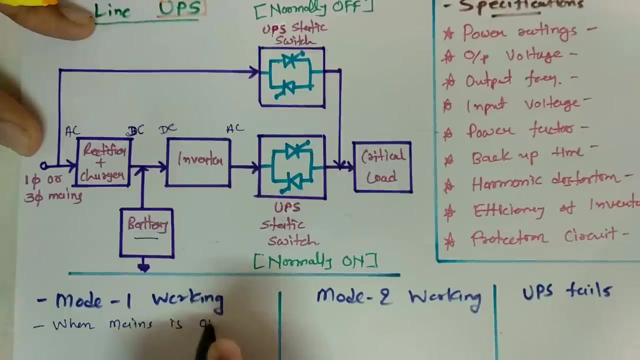 switch that is normally on and this static switch that is normally off. so let us try to understand how this circuit functions in three different modes. so first mode, that is, when mains is on. so mode one working, where condition is when mains is on. so this is what mains means: input that is available. 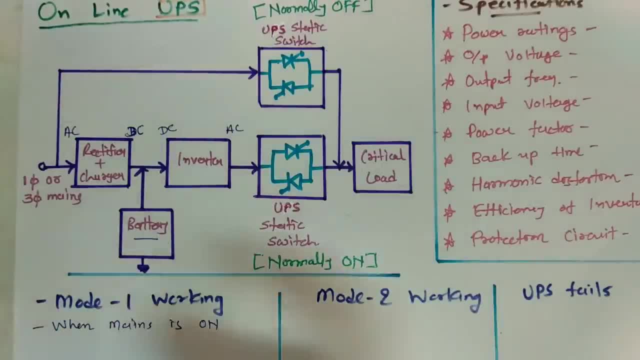 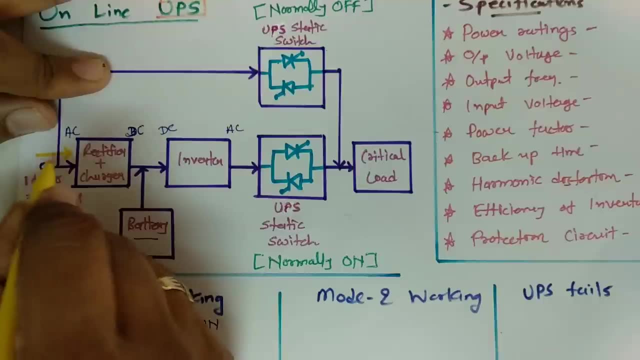 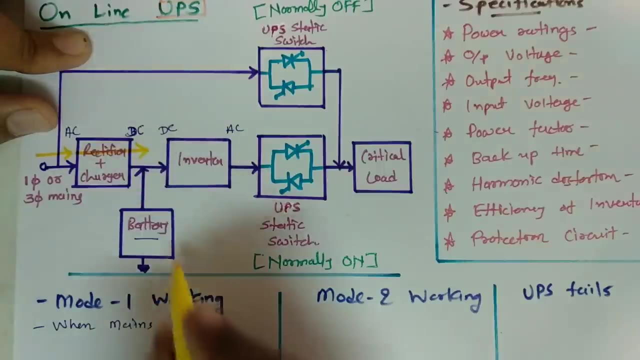 so at that time, what happens inside? so when mains is on, at that time this three phase or one phase signal that is passing through rectifier and that is what translated by ac to on DC, and that signal is given to battery to charge the battery. so here, charging. 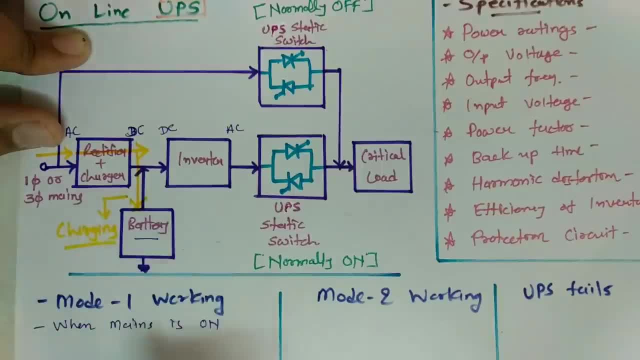 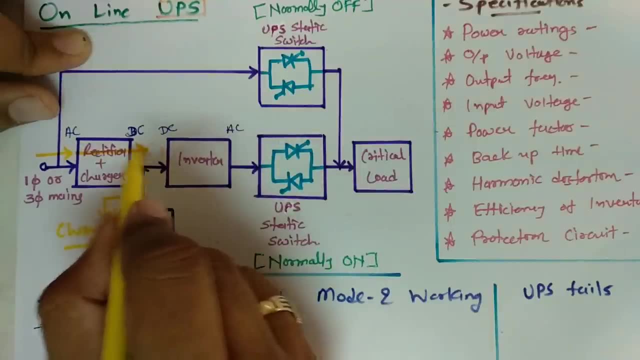 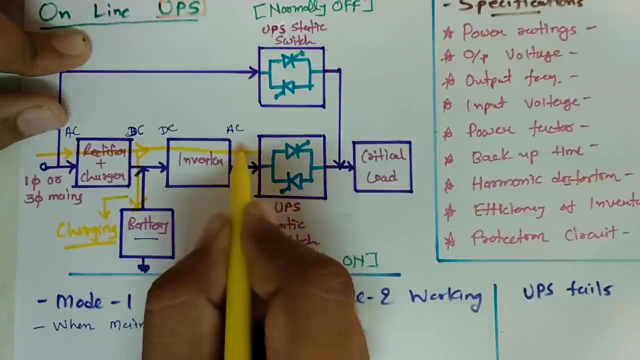 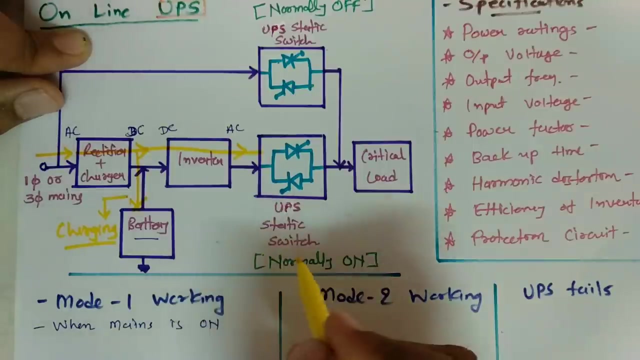 it is happening. so here charging is happening and this main signal, that is what translated to a, translated to DC from AC by rectifier and that DC again will be given to inverter and that will be resulted into AC and in this mode normally on, switch is normally on. so here this signal will be delivered to. 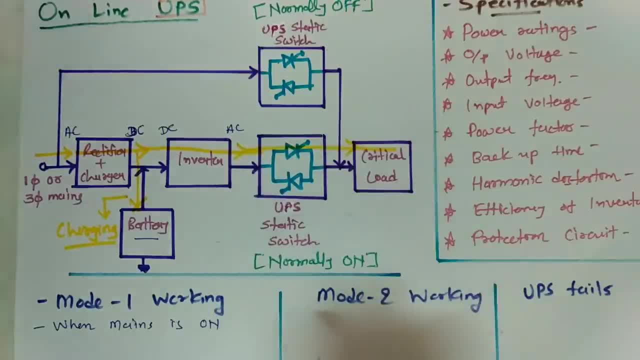 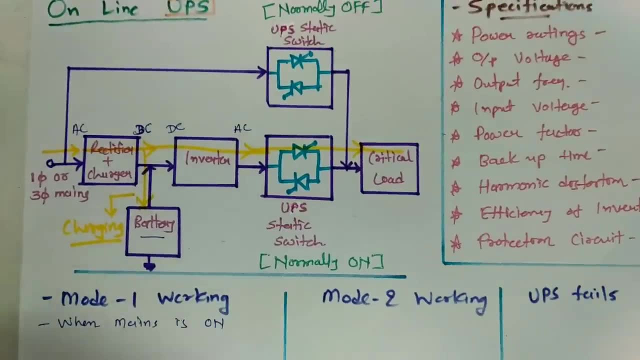 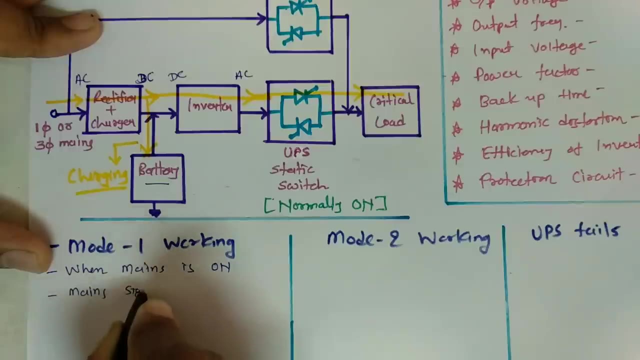 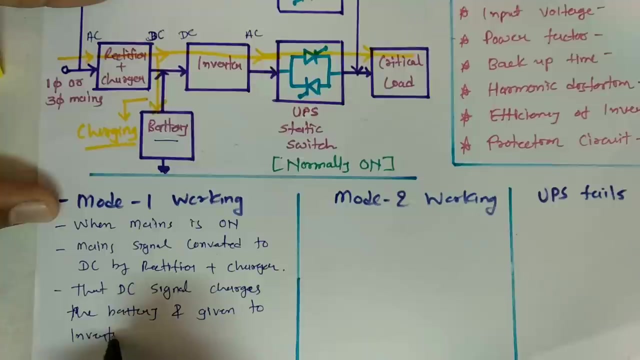 the load due to this switches on. so that is how this mode functions. so mode one, that is what when mains is on? so at that time mains sequence signal converted to DC by rectifier plus charger. so this is what. the first thing that is happening then that DC signal charge charges the battery and given to inverter. so this main signal. 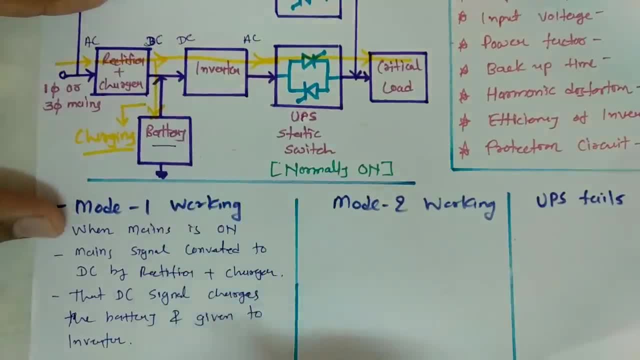 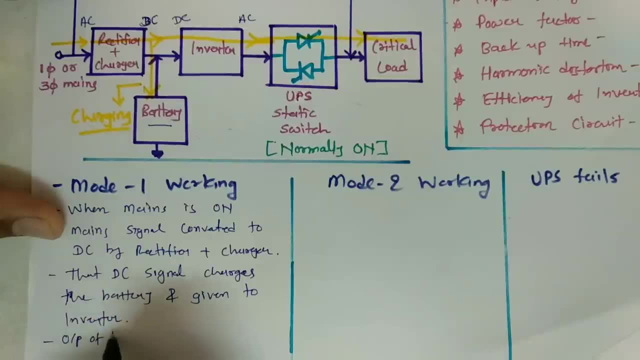 that is charging the battery as well as it is given to inverter. So this is the main signal: that is charging the battery as well as it is given to inverter And output of inverter given to load. Why output of inverter is given to load. 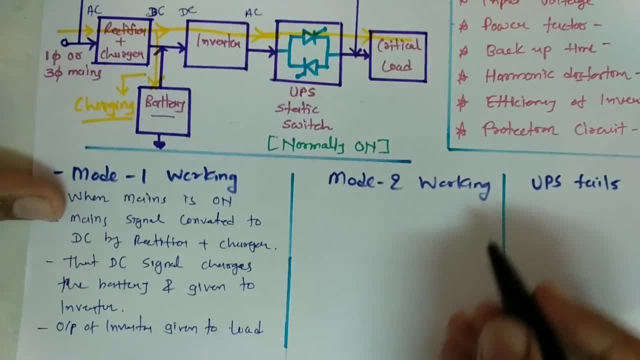 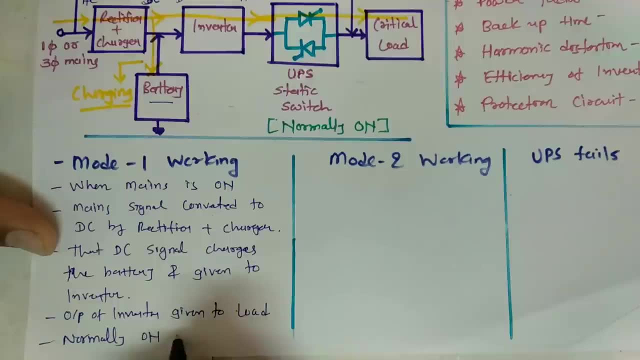 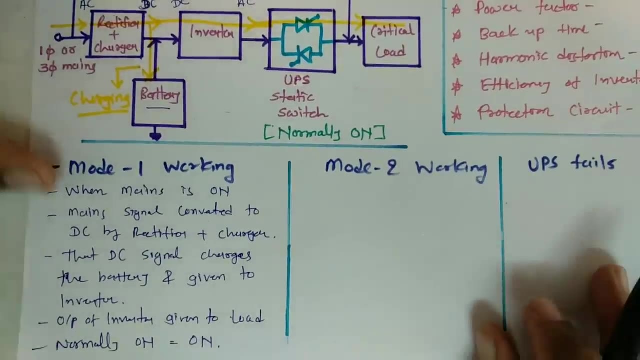 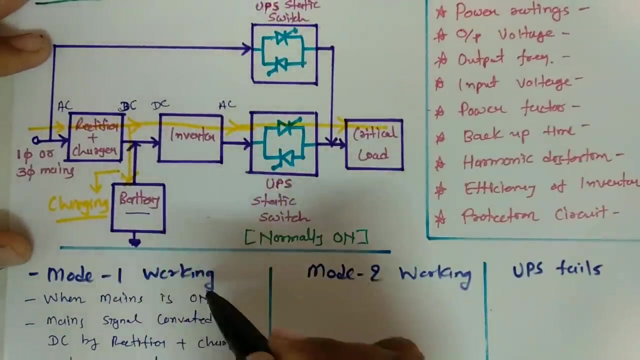 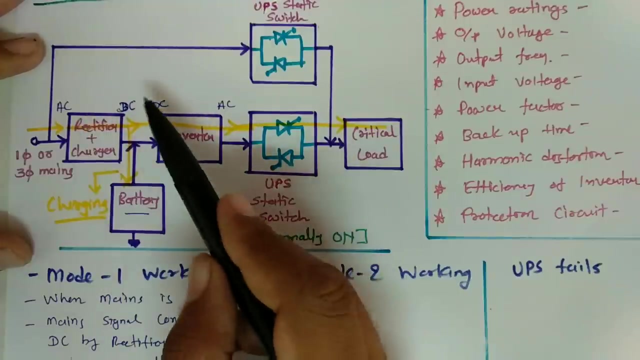 The reason is: switch normally on. switch is on, Normally on, switch is on. That's why this signal will be delivered to the load. So this is how first mode is working. again, in first mode, where mains is on one phase or three phase AC signal that will be translated into DC by rectifier, that same signal will 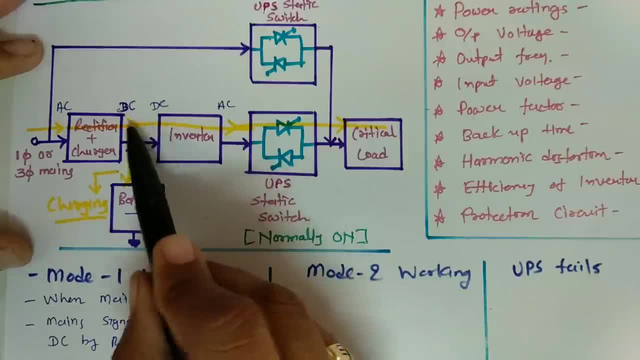 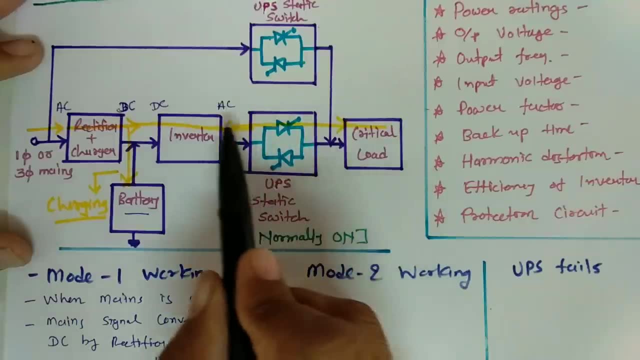 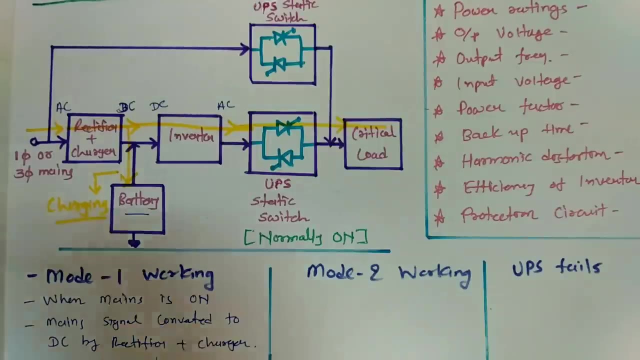 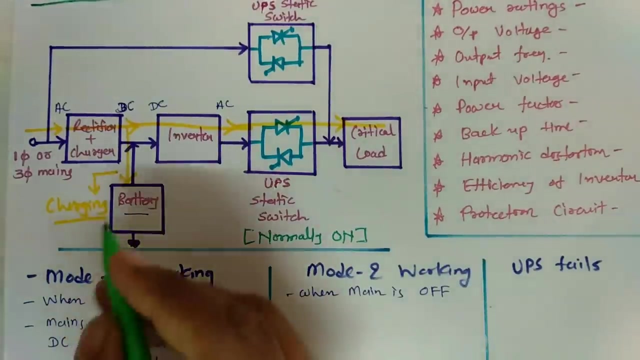 be charging battery and that signal will be given to inverter to convert that DC into AC again. Okay, Normally on switch is on, so that signal will be delivered to the critical load. now second mode of operation. so second mode is when mains is off. when mains is off means power supply. 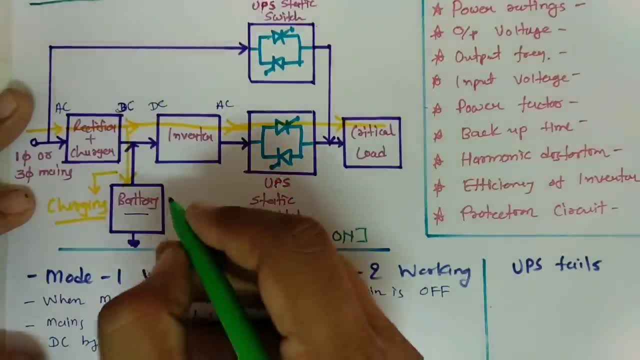 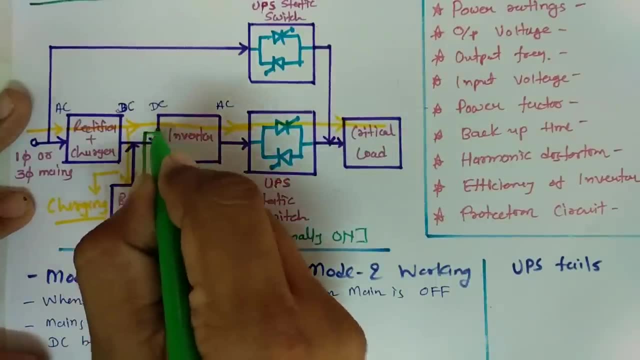 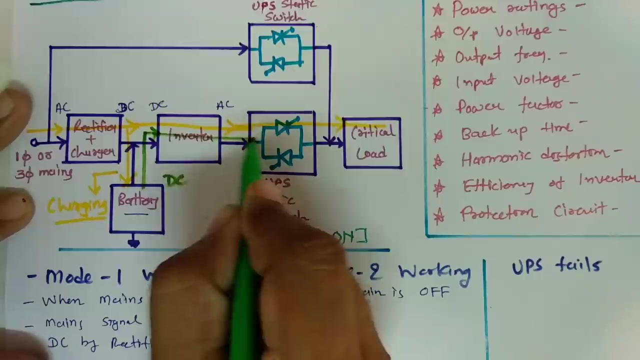 is not available. so when power supply is not available, at that time battery will provide backup to the critical load. So in this case, this battery that is giving supply to the load via inverter. so this is what DC signal that is there with battery that is getting translated into AC by inverter. 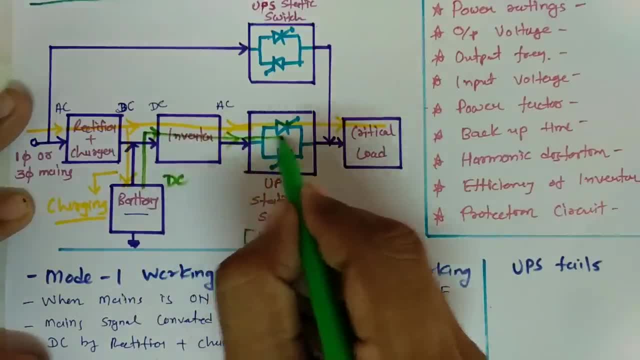 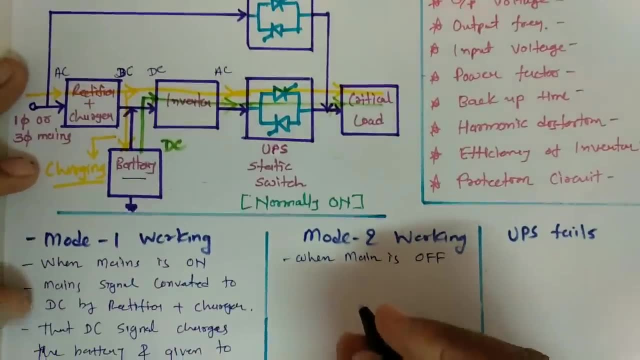 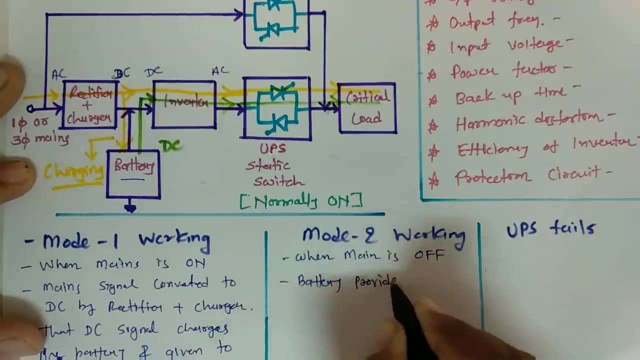 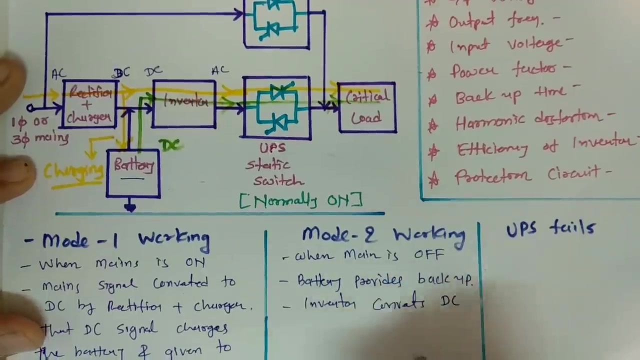 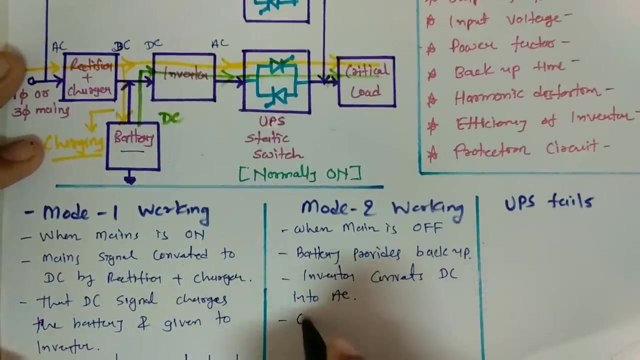 and this, normally on switch, is on. so ultimately now that will be delivered to the critical load. So when mains is off, Battery provides backup, then inverter converts DC into AC and output of inverter will be AC. Okay, So this is how first mode is working. again in first mode. 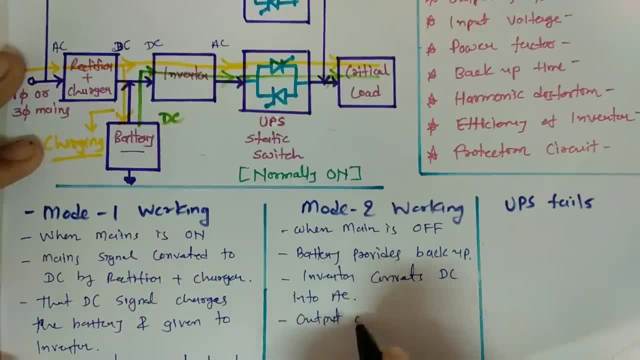 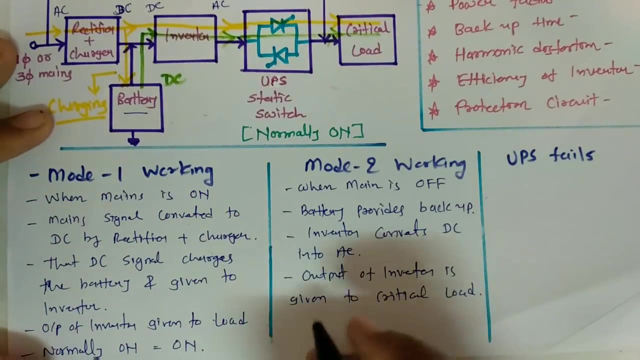 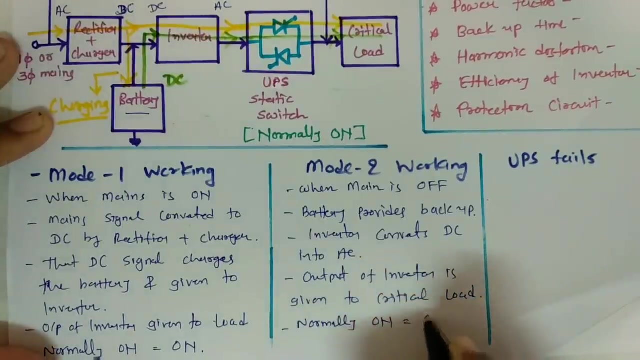 So this is how first mode is working, again in first mode. So when mains is off, An inverter is re plugged, or clearly visible ours, then it will be a normal power step. Okay, Leonardo, a very simple method of compressing an inverter. 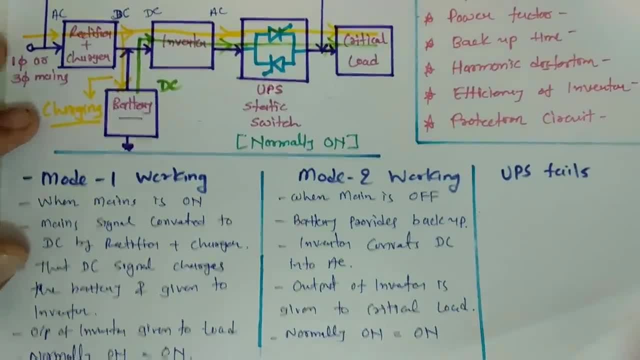 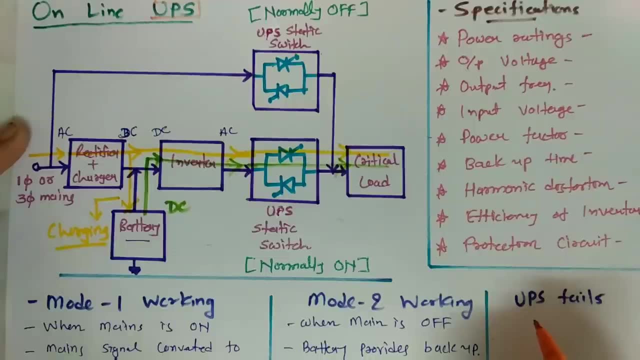 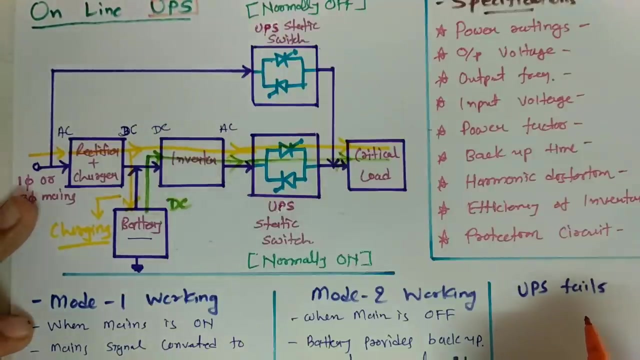 Okay, integral load. Now in third mode of operation. what if this UPS is getting failed? So in third operation? what will happen? So in third operation case is, what if UPS is getting failed? So in case of this circuit, if this circuit which I have placed in box, if it is getting failed, So what? 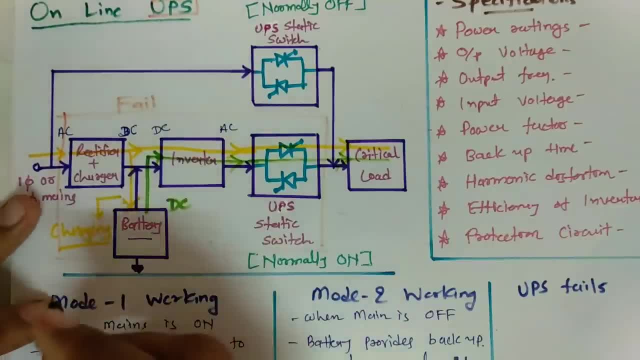 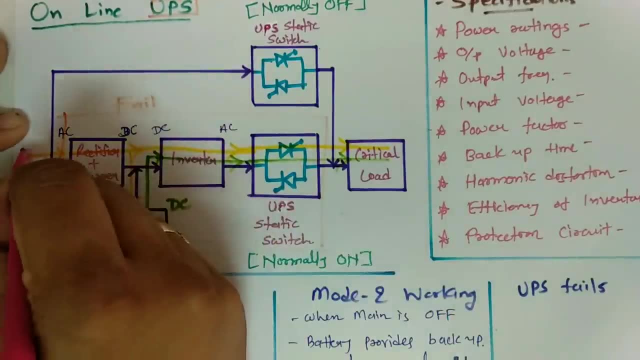 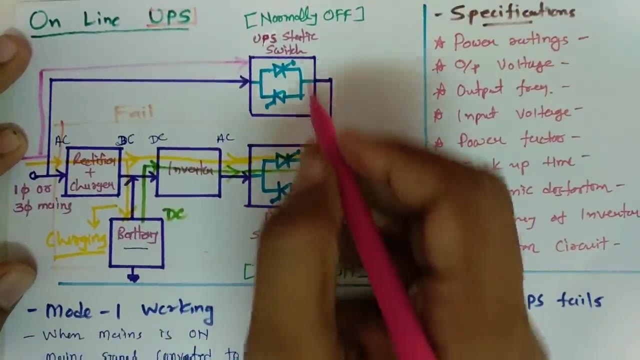 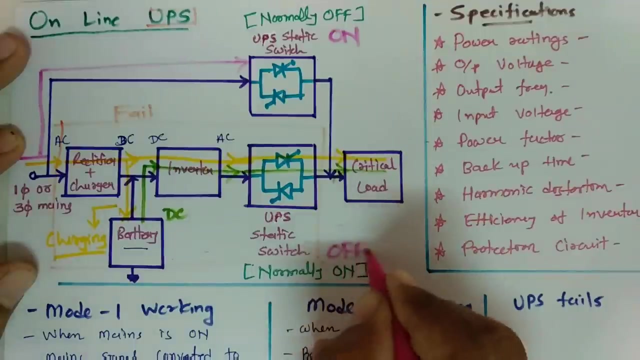 will happen. So for that there is one condition here, and in that condition here, three phase supply, that is what passing over here, and this normally off switch That is getting on, and this normally on switch that is getting off. So now the signal will pass. 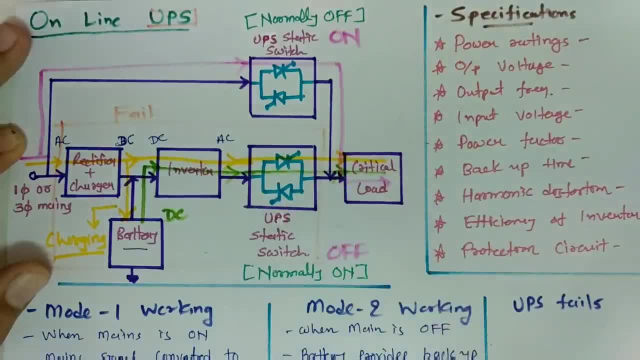 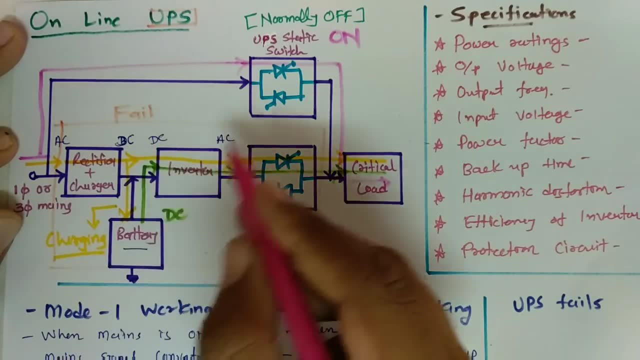 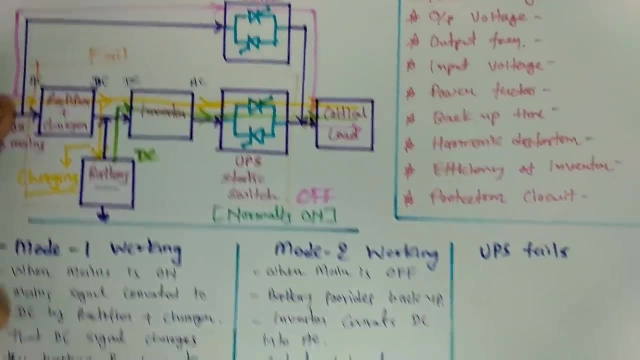 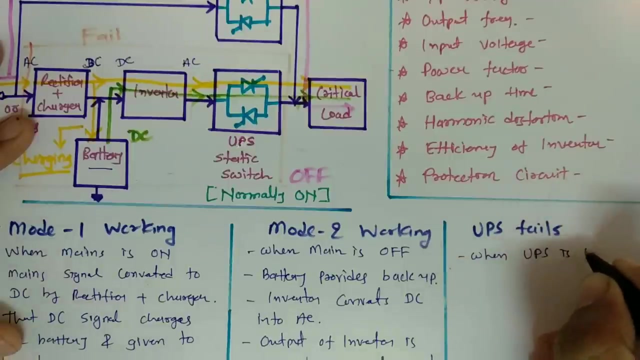 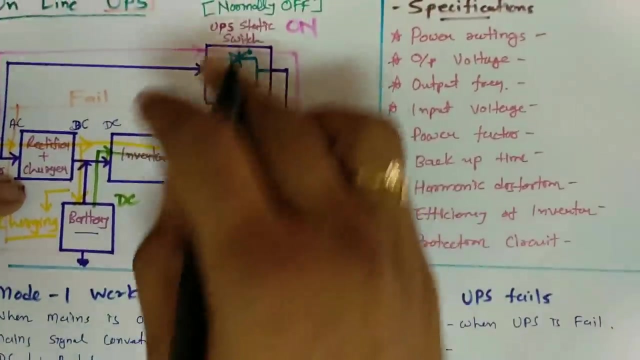 through this switch and it will be delivered to the critical load and during that time we can have a maintenance of this circuit. So during that time we can have a maintenance of this circuit. So what if UPS is getting failed? So when UPS is fail, at that time switches are getting triggered, so normally off is. 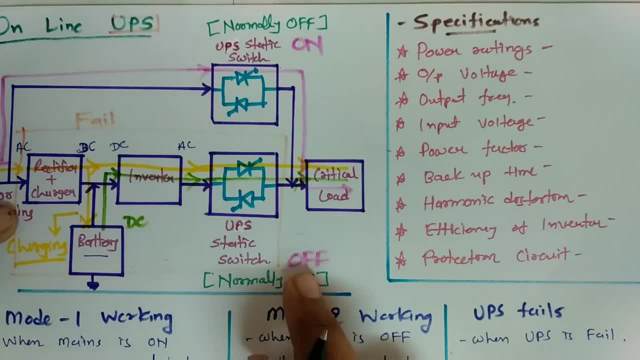 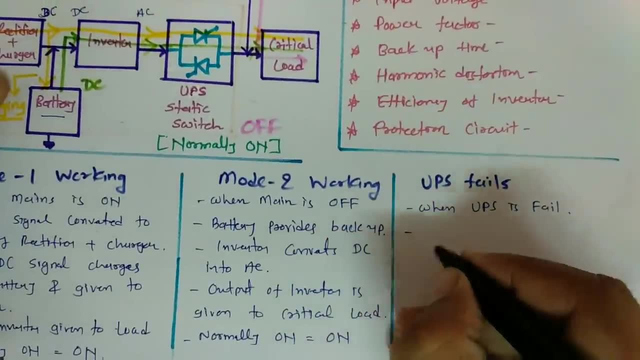 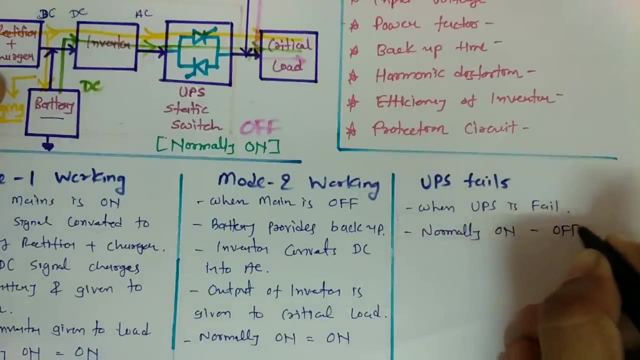 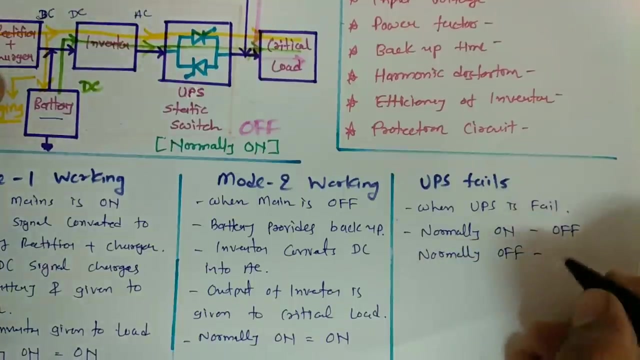 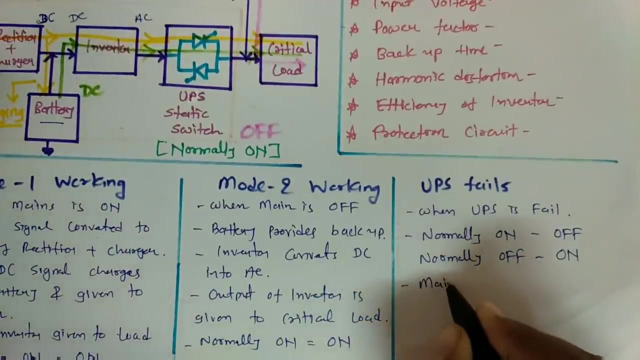 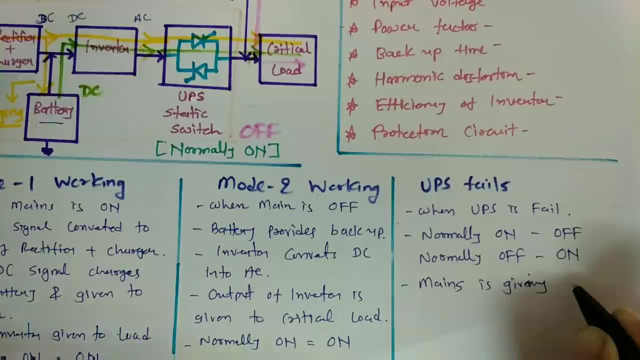 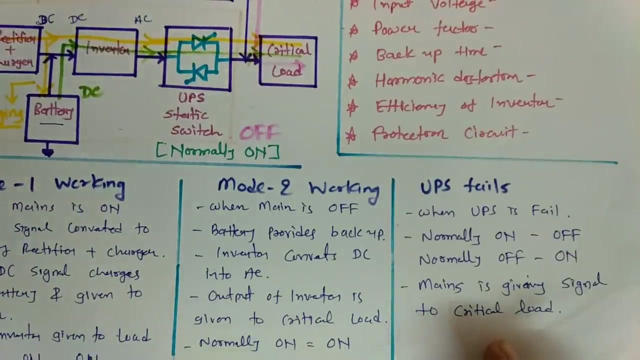 getting normally on and normally on is getting normally off. so this signal now that will pass through this path and it will be delivered to the load. so normally on switch that is getting off and normally off switch that is getting on. so mains is giving signal to critical load. in this situation, mains is giving signal to critical load. so 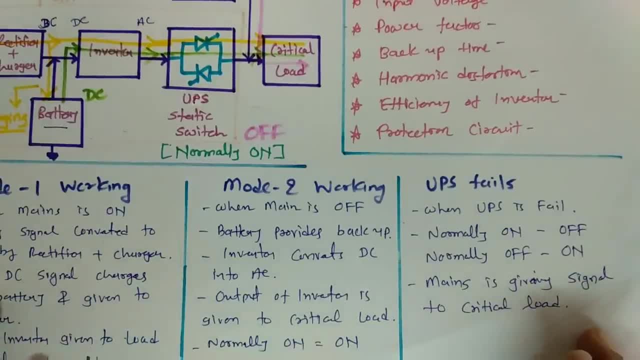 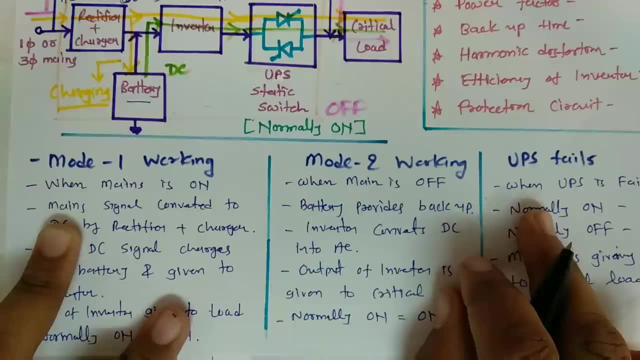 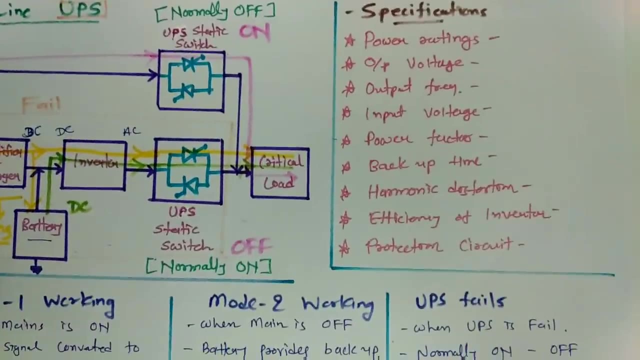 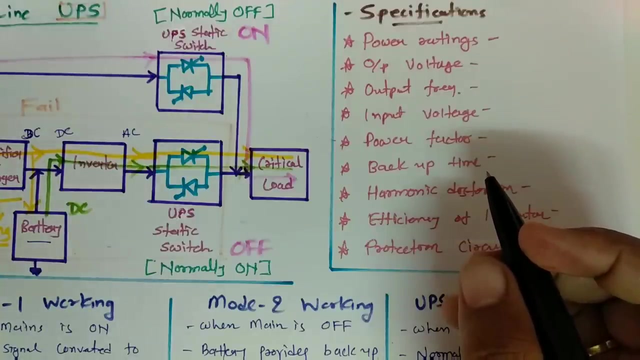 this is how UPS is, having three different modes. first mode is when mains is on, second mode is when mains is off and third mode is when UPS is failed. now I'll explain few specifications which we need to understand before we buy any UPS. so I'll explain: what are the ratings, which is there which? what are the specifications? 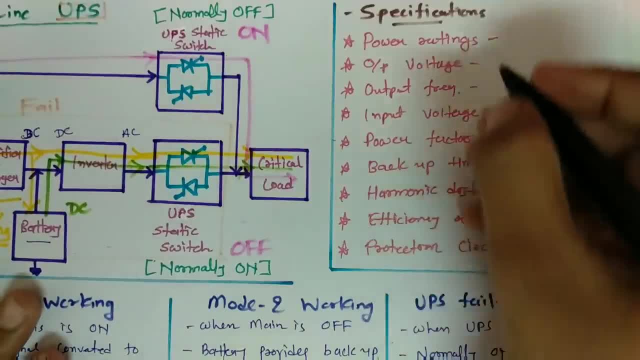 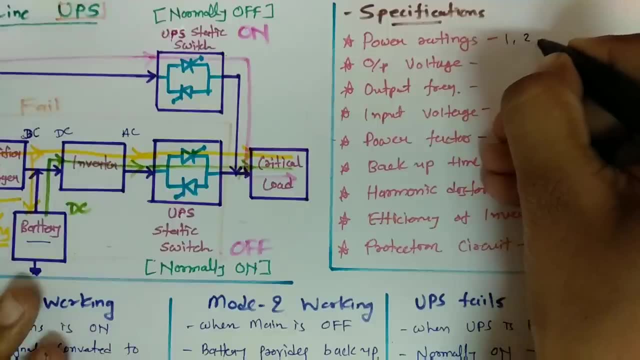 which is there with UPS. so power rating of UPS that is available by 1 kilowatt ampere, 2 kilowatt ampere and 5 kilowatt ampere. so this is the power rating: 1 kilowatt, 2 kilowatt, 5 kilowatt ampere that is available with UPS output. 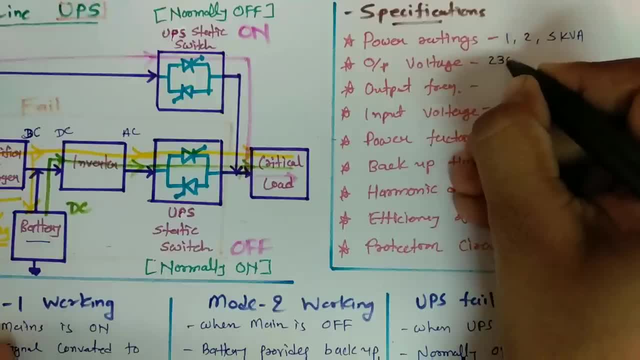 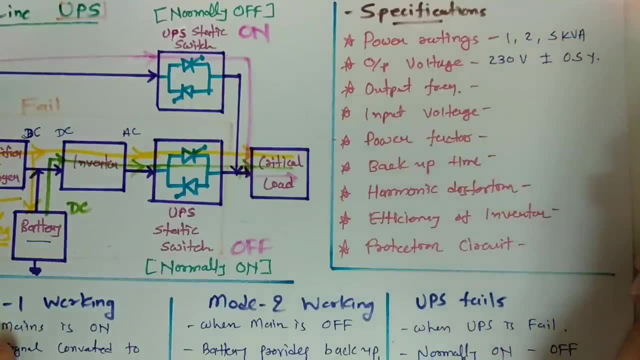 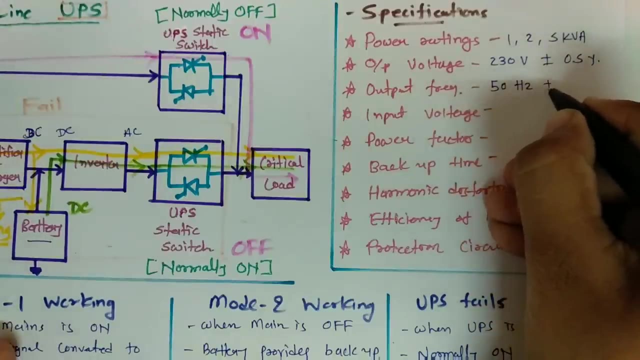 voltage in India available with 230 volt age plus or minus 0.5 percentage output voltage in India available with 230 volt age plus or minus 0.5 percentage output. output frequency: that is available by 50 Hertz plus or minus 2 Hertz input voltage range. 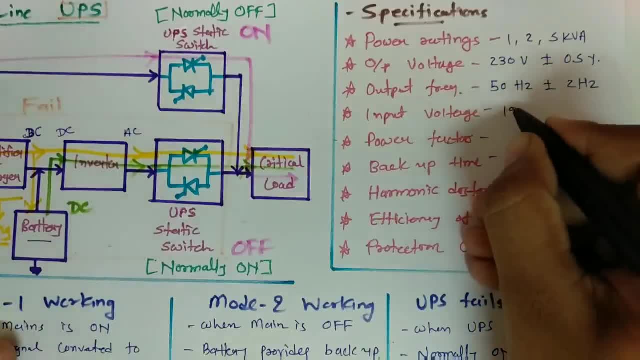 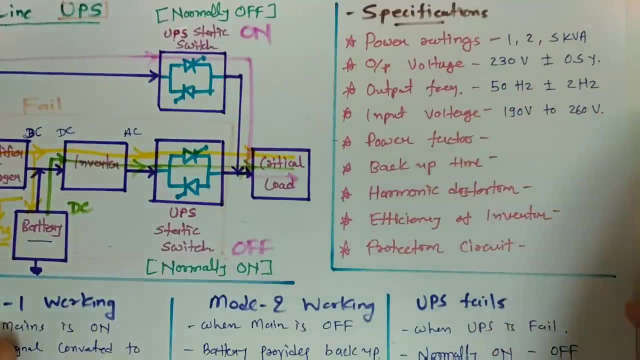 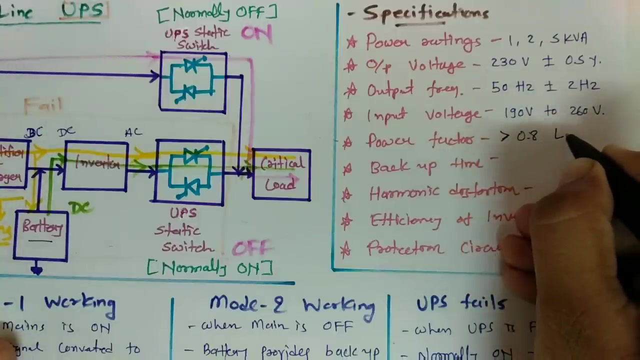 voltage range that varies from 190 volt to 260 volt. so if input varies in this vicinity, there is no problem. it will be providing steady voltage. as we have seen, at output voltage and output frequency, power factor that is greater than 0.8 and it is being utilized as lagging, and that too, because of inductive load. so 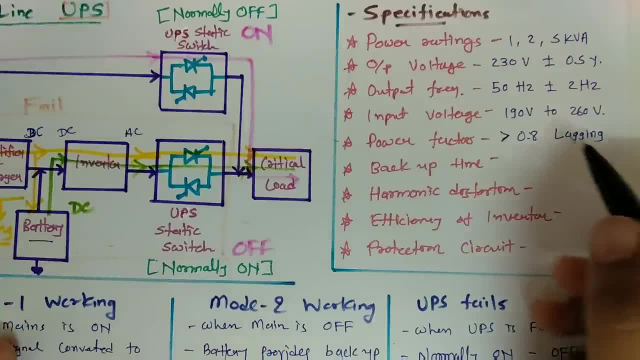 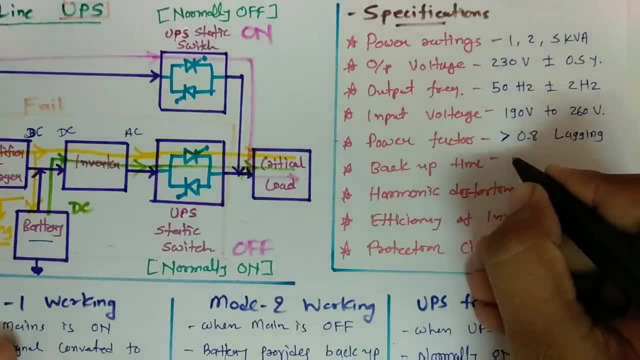 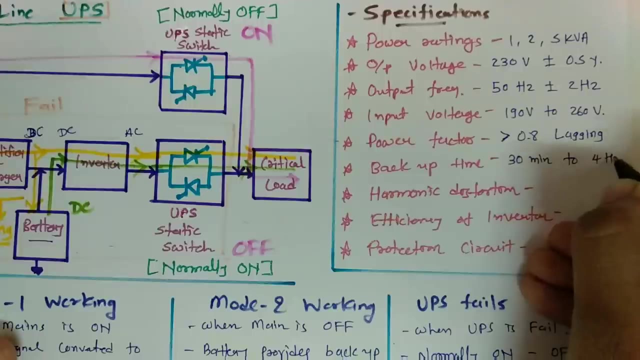 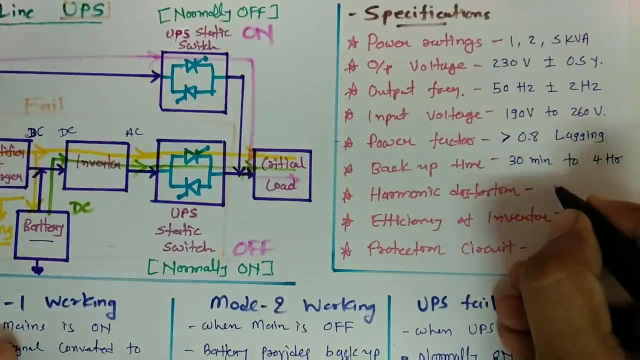 lagging power factor that is been utilized due to inductive load and it should be greater than 0.8. backup time available with this now online UPS from 30 minutes to 4 hour. so these sets of UPS available. harmonic distortion so that, should that, will be available with less than 5 percentage efficiency of this. 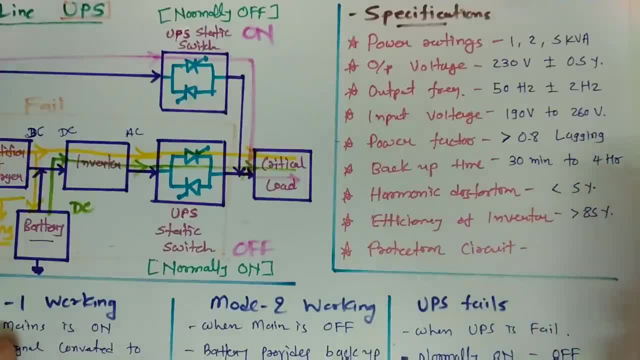 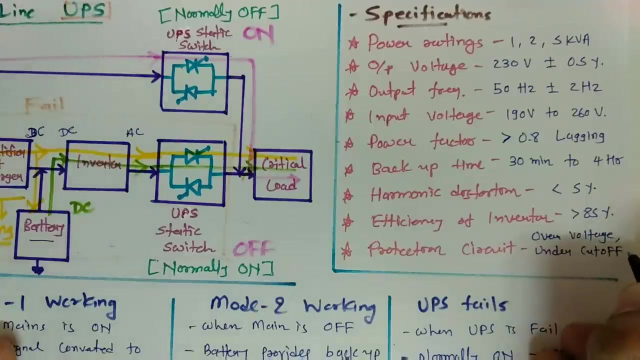 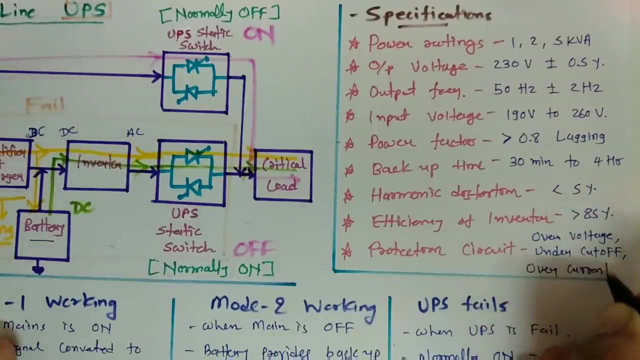 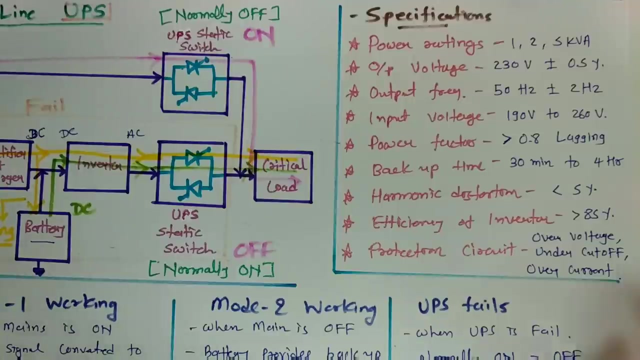 set of UPS that is greater than 85% and there are two different protection circuit which is required. one is over voltage and under cut off, protection Over voltage, under cut off and third is over. current protection circuit is required for online UPS. So these three different circuits which is required to have a protection of online UPS. 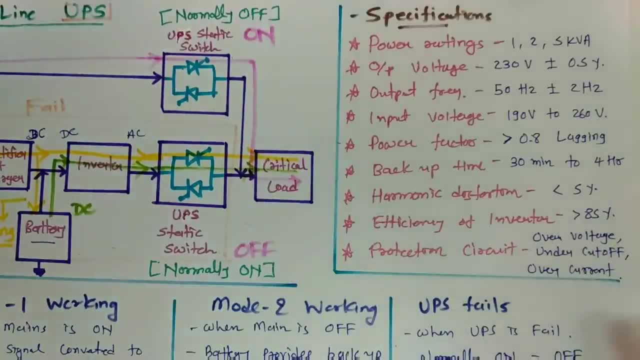 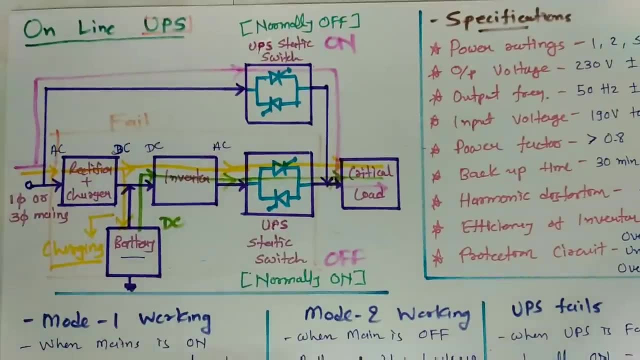 over voltage, Under cut off and over current protection. So these are the basic specification which is available and this is how online UPS functions. Thank you so much for watching this video. If you like this video, then press like button and if suggestions are required, give suggestions. 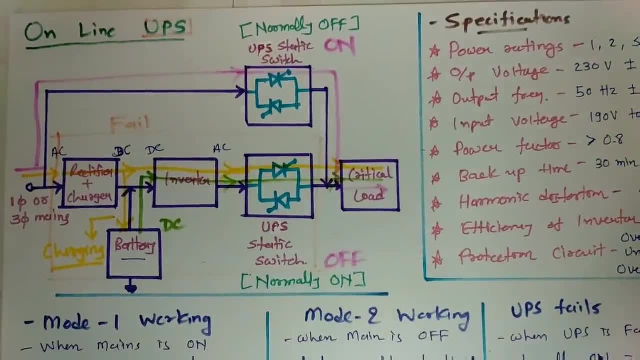 in comment. definitely, I will get back to you. Thank you so much for watching this video.